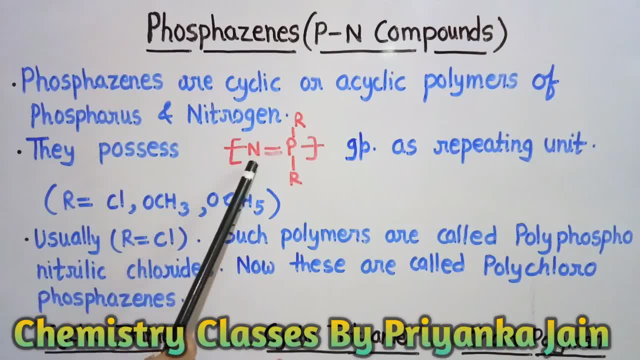 double bond. there are partial double bond characters between all the anion, phosph, nitrogen and phosphorous atoms. We will study it about it later. Firstly, we see these as presented in the repeating unit and the phosphagenes are the monomer. these are the polymers of. 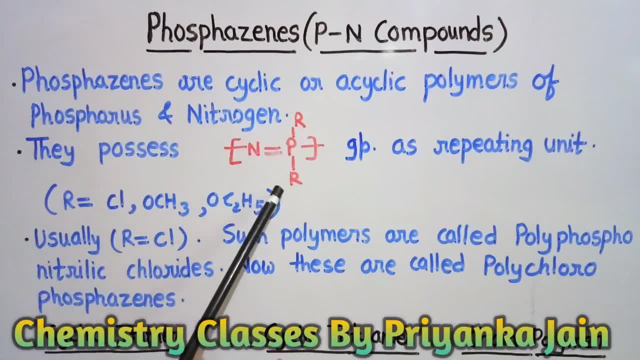 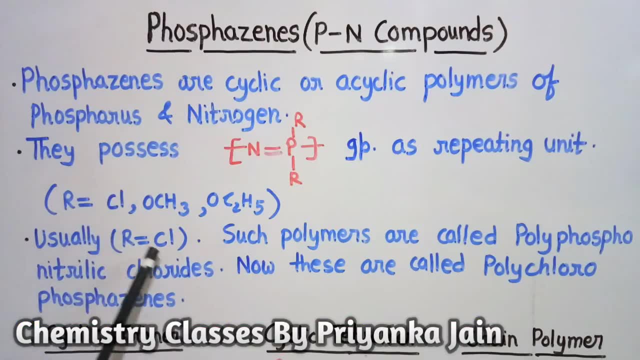 these monomer units Now here, R group. this R group may be chloride, this may be methoxy or this may bethoxy, and such polymers are known as the poly phosphonitrile chlorides, and nowadays these are also known as the polychlorophosphate genes. so this is the 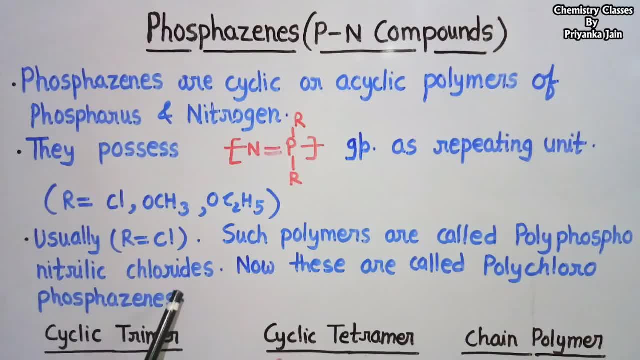 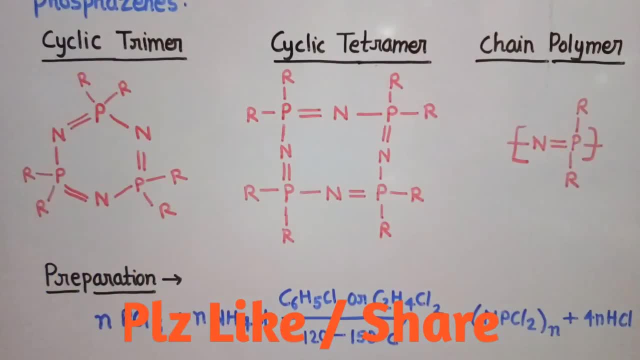 old name, that is polyphosphonitrile chloride, and the newer days the name is polychlorophosphate genes, so phosphatines. if we see that classification of the phosphatines, phosphatines are of three types: cyclic trimers, cyclic tetramers. 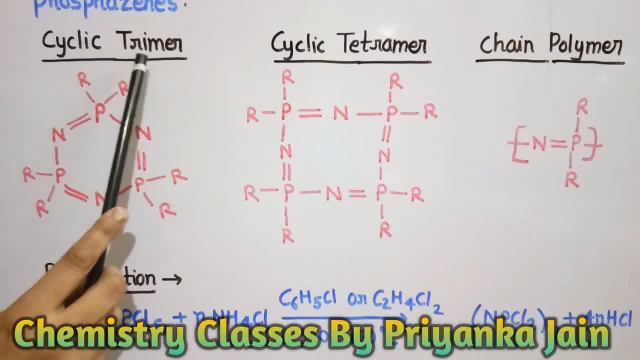 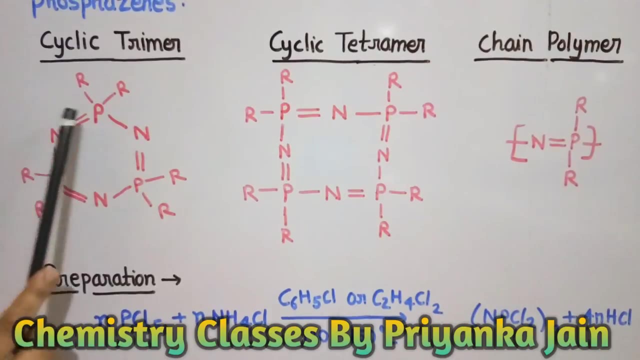 and the chain polymers. what is cyclic trimers? it means van, try means three, when there are three and PR two units present, and these are joined together to form a cyclic structure, this is called a cyclic primer. for example, this structure is a cyclic primer, and when here two chlorine atoms are present, then we will: 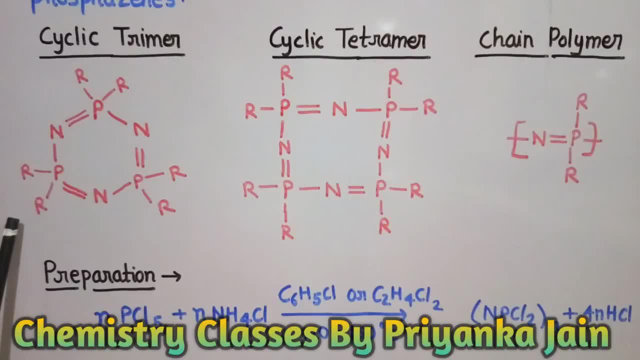 call it hexachloro cyclotriphosphate, hence any maybe group present here. the R may be any instead of chloride group. now we see the structure of cyclic tetramer. when there are four NPI, two units present, then that will look like this: this is structure will be formed. that will be. 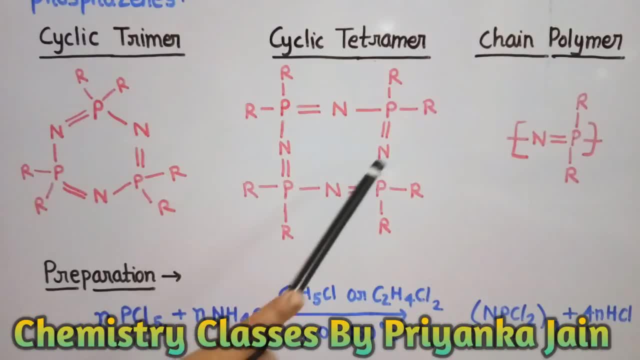 called the cyclint entomology captain and the another structure may be chain polymer. when these NPI two units are present repeatedly but they are not from any cyclic structures. there are present like a chain reason is chain polymer chain, then this is called a chain polymer. now we see the preparation of the phosphagenes. phosphagenes: 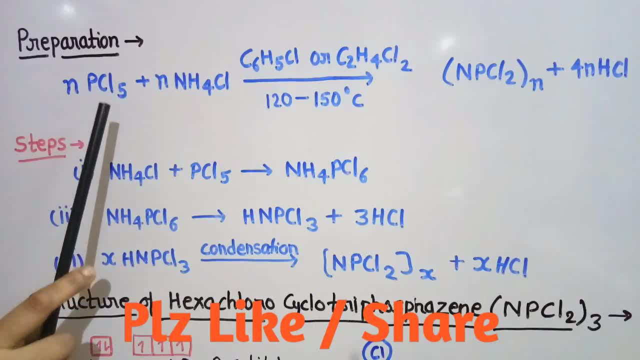 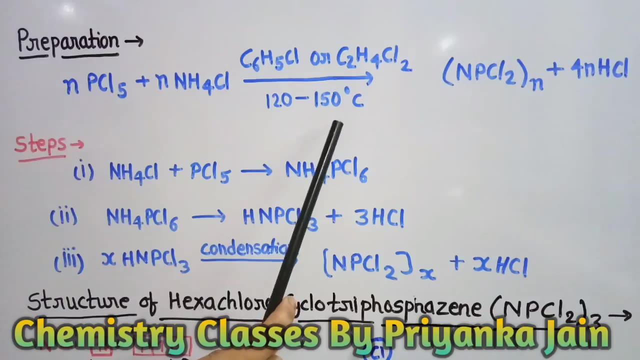 are prepared by the condensation of phosphorus pentachloride with the ammonium chloride, and this reaction is catalyzed in the presence of chlorobenzene or dichloroethane, and at the 120 to 150 degree centigrade. as a result of this, phosphagenes formed and the hydrochloric acid. 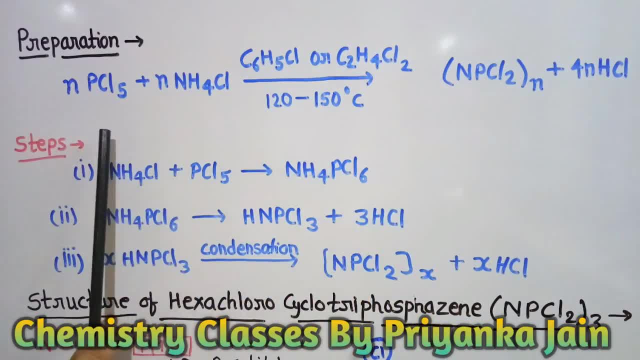 is formed under the controlled conditions. the main products are the cyclic trimers and cyclic tetramers. if we see the steps, this reaction takes place under the three steps. the first step is the reaction of this ammonium chloride with phosphorus pentachloride and, as a result of this, a 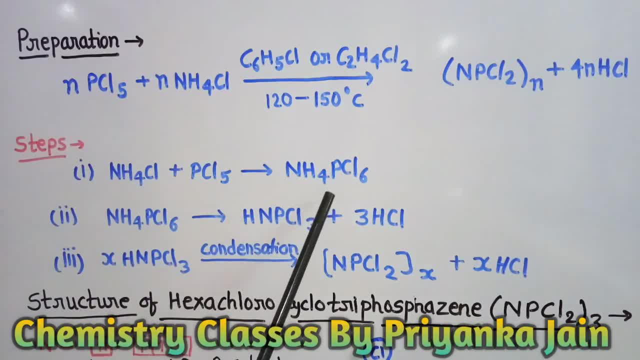 condensation product. the second step: this dissociates and forms NHpCl3 and three molecules of SCL. now this NHpCl3 H molecule of this NHpCl3 condensed together and forms phosphagenes with X units, X basic units or monomers: NHpCl2 and NHpCl3. that is the most complex molecule that exists and such molecular 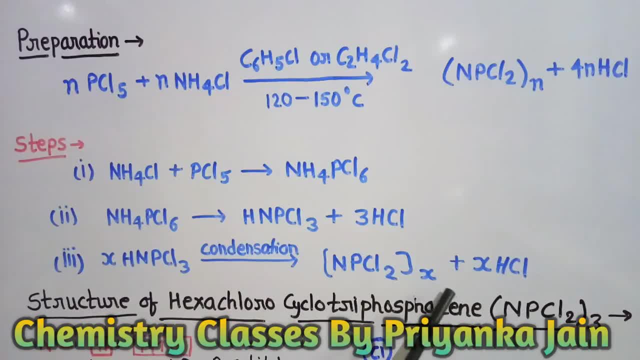 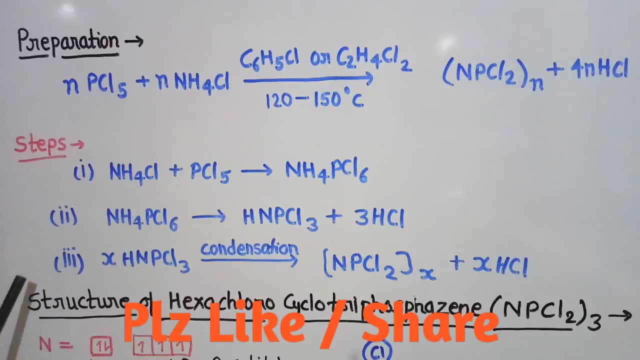 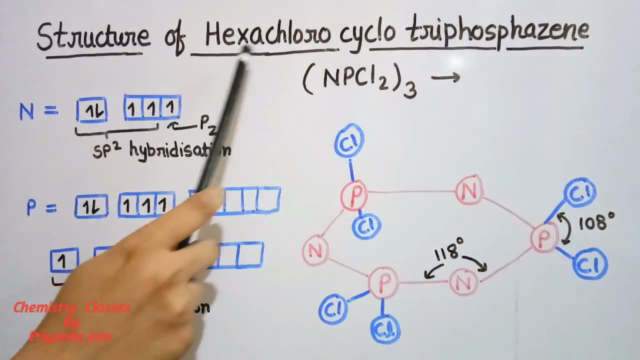 X and X molecules of hydrochloric acid are formed, and this is a very important reactions. several times, questions are asked on the these reactions. now we see the structure of one of the most important type of phosphagen, that is, hexachloro cyclotriphosphazine. the formula of it is npcl2- whole thrice and 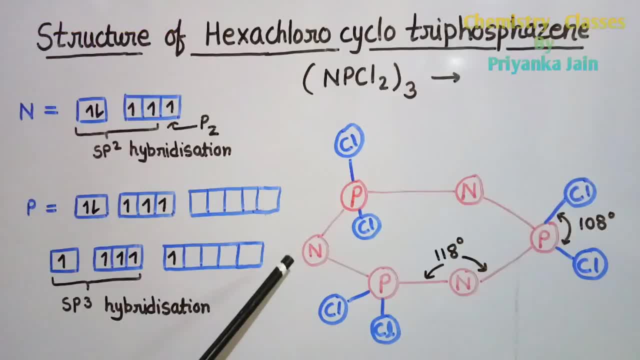 this is the structure of this compound. actually it is a planar structure and this is a six membered ring of alternative nitrogen and phosphorus. it means the nitrogen are and phosphorus are present alternatively in a single plane, same plane, and two chlorine atoms are attached to each phosphorus atom. now 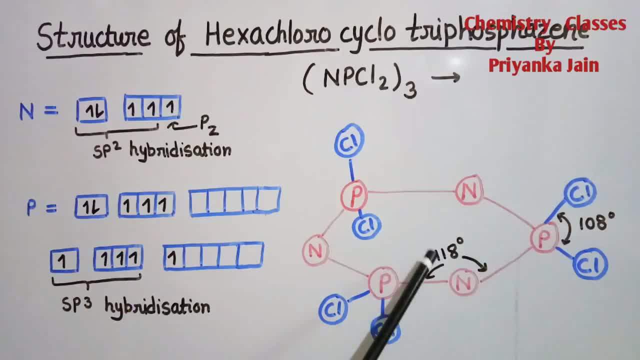 you can see the angle of PNP bond is 118 degree and the angle of CLP, CL. this angle is 108 degree. this molecule is planar and we have shown that there is a double bond and a single volt and dilative single and double bond, but in actual there is no. 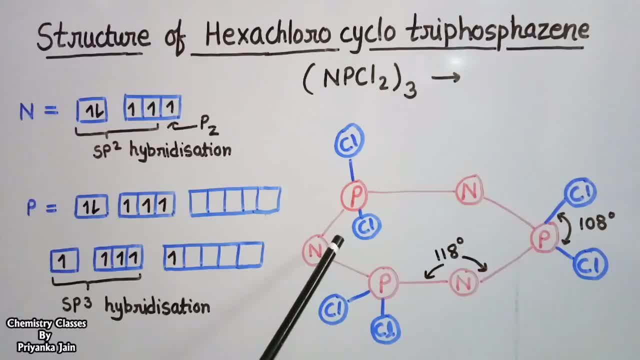 alternating double and single bond. all bonds are same and all bonds have partial double bond character and this is due to the resonance. it means it is a resonating structure, as in the case of benzene. but there is somewhat difference from the benzene. it involves the p orbital and the d orbital and it involves there is also difference in the 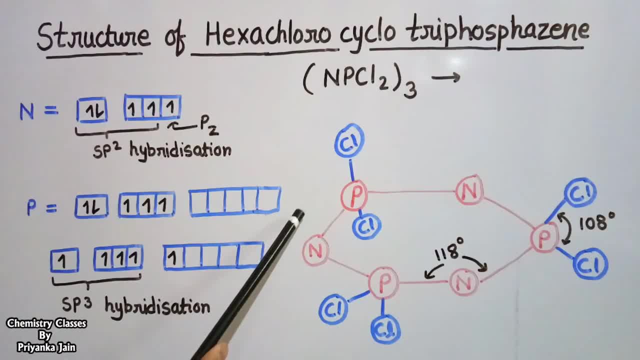 hybridization state and further here. in the case of benzene, two carbon atoms are involved, but in this case one phosphorus and one nitrogen atoms are involved. if we see the hybridization state of nitrogen and phosphorus. in the case of nitrogen you can see it possess five electrons. 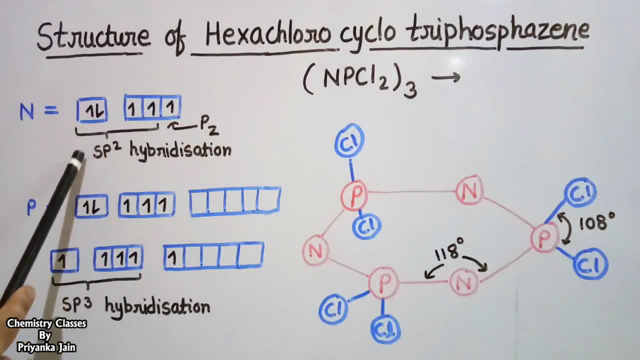 five valence electrons and it does not have d orbital, and the s and two p orbitals undergoes sp2 hybridization to form three sp2 hybrid orbitals, while the pz orbital remains as it is. if we see the hybridization state of phosphorus, it also possess five valence, so the delocalization. 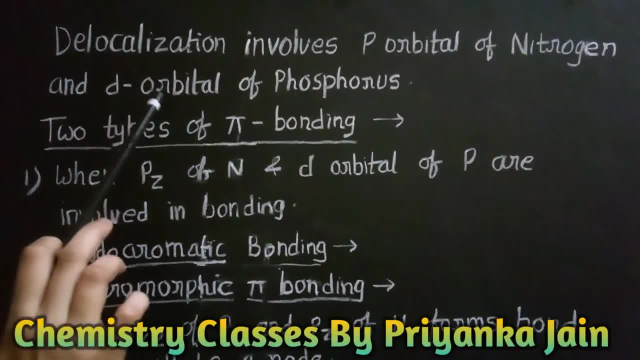 involves the p orbital of the nitrogen and the d orbital of the phosphorus. we can also say a p? d type of bond is present in the case of phosphazine and there may be two type of pi bonding in this case. the first type of pi bonding may be when the pz orbital of the nitrogen and the 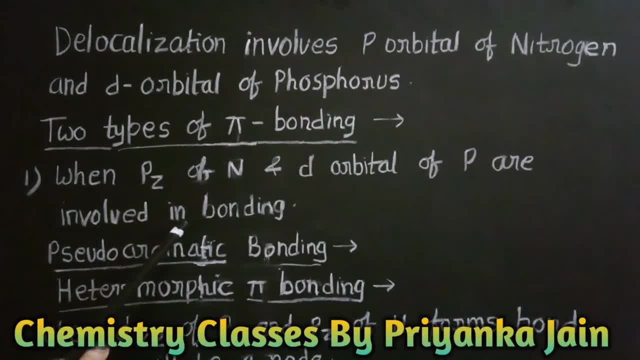 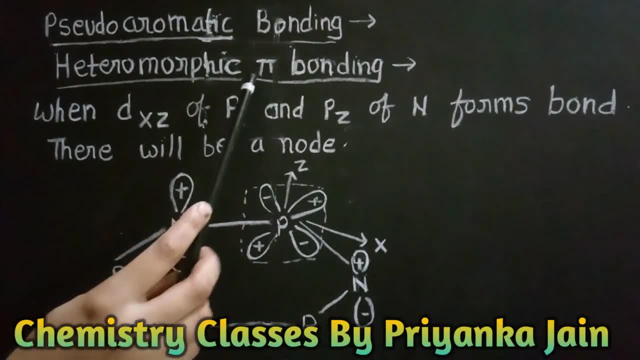 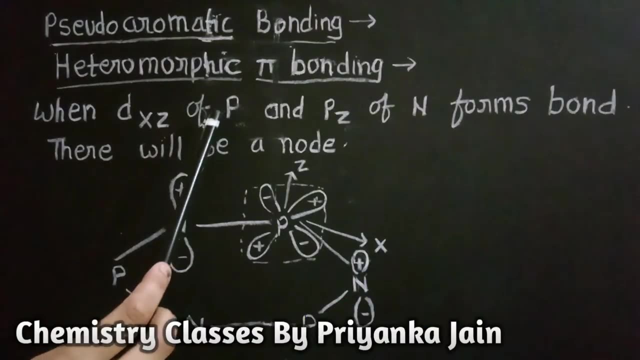 d orbital of the phosphorus are involved in the bonding, and this type of bonding may be of two types. the first type of bonding may be hydromorphic pi bonding, or it is also known as the pseudo ían type of bonding, and this happens when the dxz orbital of the phosphorus and the pz. 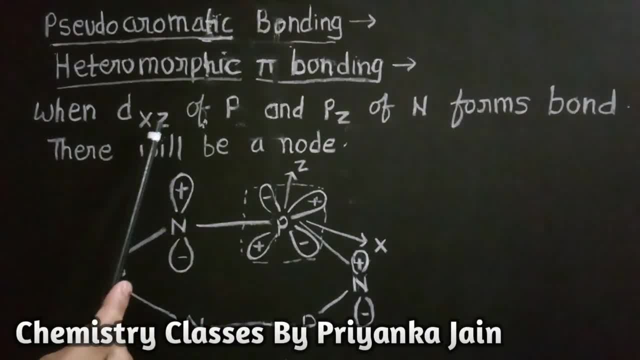 orbital of the nitrogen forms the bond that is pi bond, and their symmetries does not match, so there will remained, in this case, suppose this is that profile. this is the picture that is showing the hydromorphic pi bonding and this is the nitrogen's pz orbital. 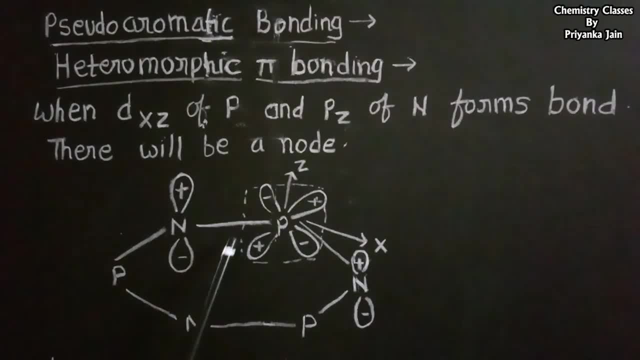 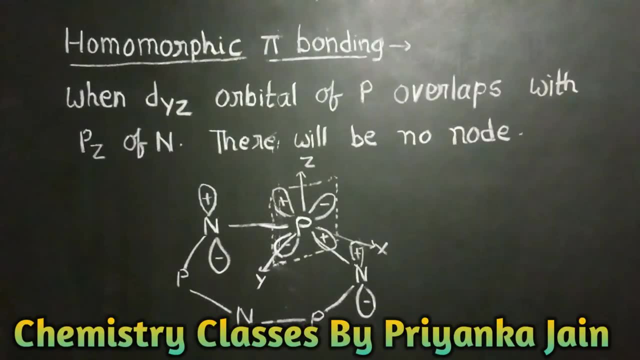 and this is pz orbital of another nitrogen, and here this is the dxz orbital of the phosphorus, and these are phosporous time-promotion and these are forming bond. now you can see their symmetries are not matching, so there will be a node. the another type of bonding is the homomorphic pi bonding. 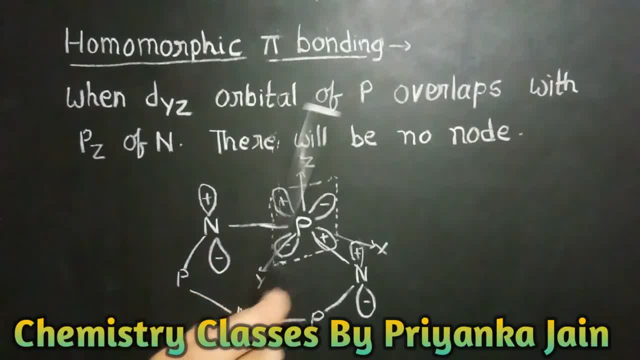 when the D Y Z orbital of the phosphorus overlaps with the P Z orbital of the nitrogen and their symmetries match. so in this case there will be no node. so it is called homomorphic pi bonding and this can be shown in this picture. this: 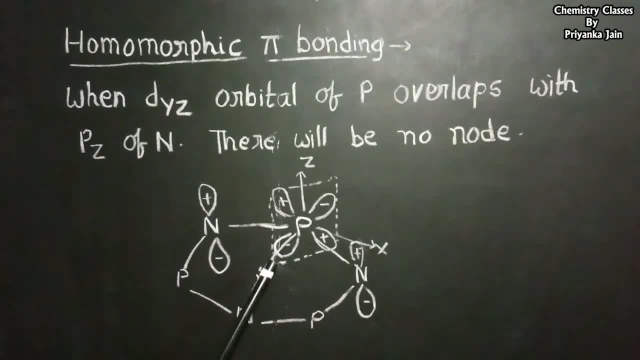 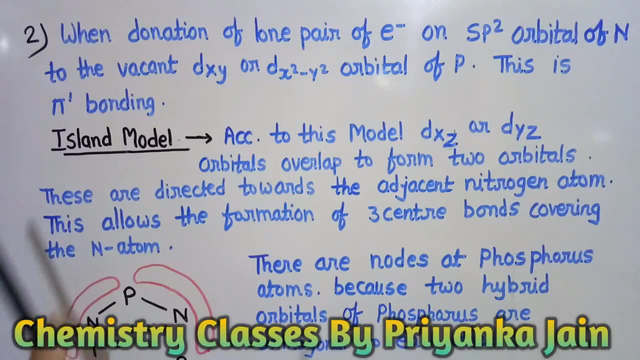 is P Z orbital of the nitrogen and this is the D Y Z orbital of the phosphorus and their symmetries are matching. so there will be no node. so it is homomorphic pi bonding. the second type of pi bonding: where happens? it happens when the donation of lone pair of electrons on the sp2 hybrid orbital of 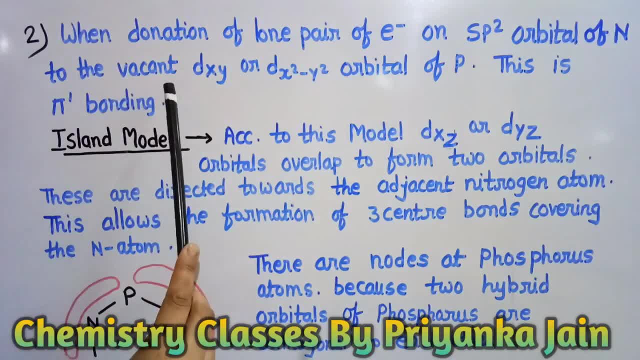 nitrogen takes place to the vacant D xy or D x squared, and the donation of lone pair of electrons on the sp2 hybrid orbital of nitrogen takes place to the vacant D xy or D x squared, minus y square orbital of the phosphorus. what happens? it means when we 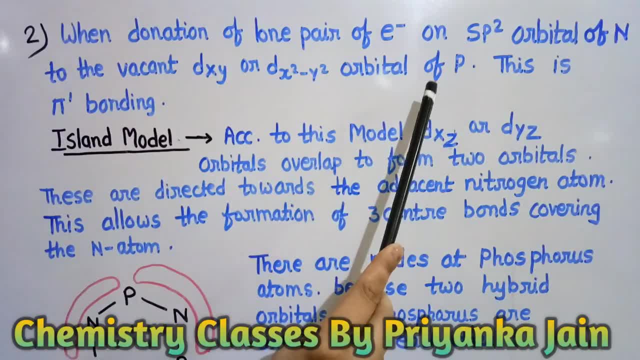 know that the nitrogen possess a lone pair of electron in its one of the sp2 hybrid orbital, and when this lone pair of electron is transferred to the vacant D xy or D x square minus y square orbital that is present on phosphorus, such type of bonding is formed. this type of bonding is known as the pi-bonding. 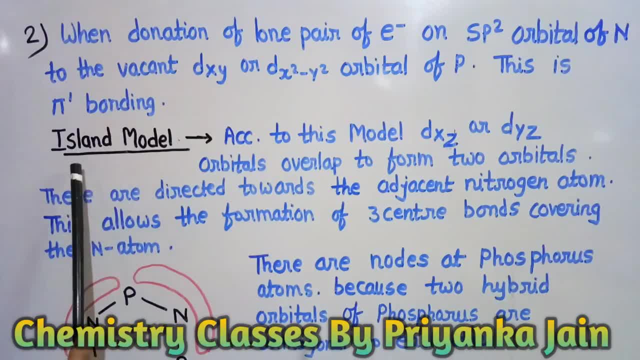 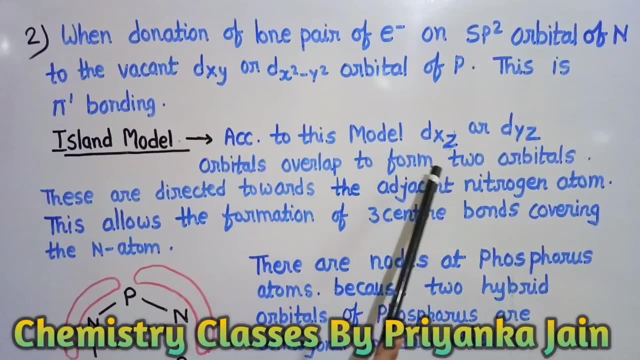 now another model has also been given that is known as the Eisschland model. Eisschland model: according to this model, that D x, z and d y z orbitals of the phosphorus overlaps together and forms two orbitals, and these two orbitals are: 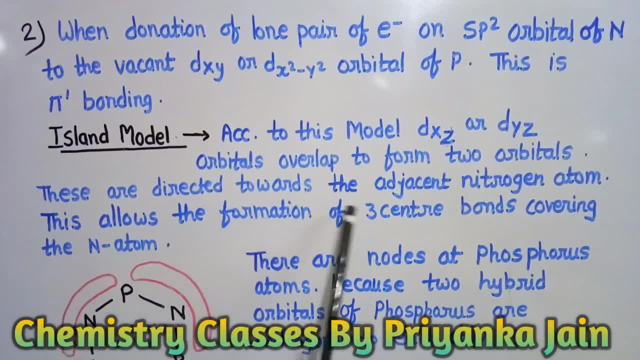 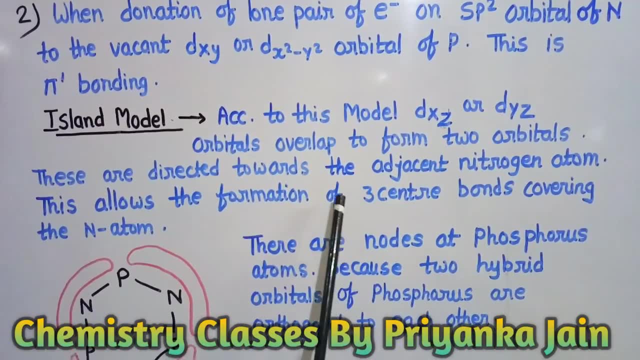 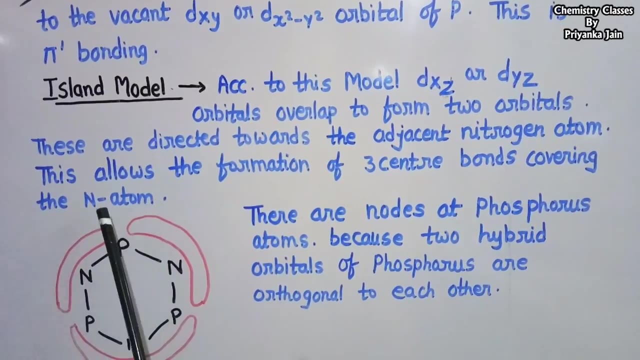 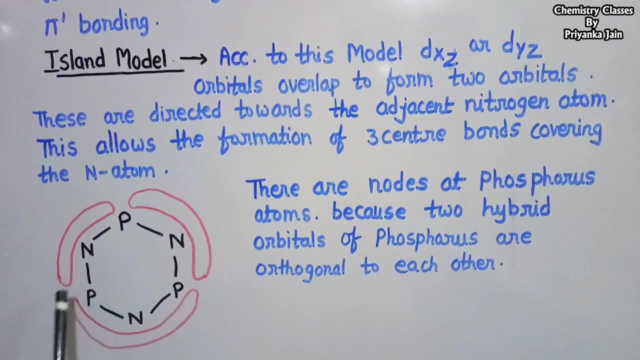 directed toward the adjacent nitrogen atoms. it means one orbital is directed toward one nitrogen atom and the another is directed toward the adjacent nitrogen atom, another nitrogen atom. in this way, this forms a three centered bond. it means it is also covering the nitrogen atom, and you can understand this with the help of this diagram. this is the iceland model. 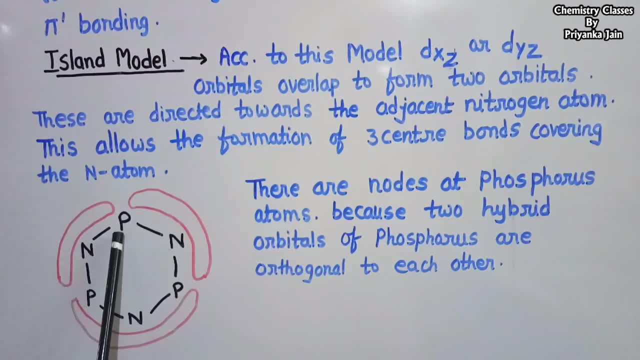 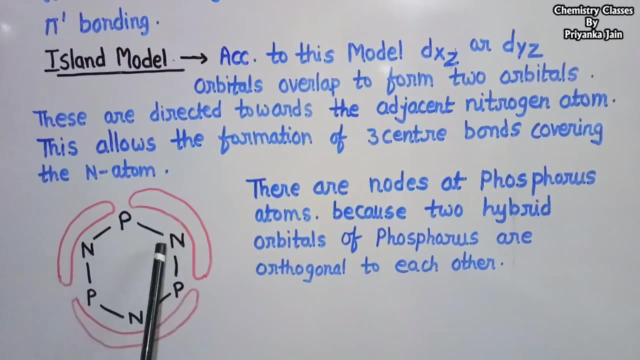 for the phosphagen and you can see, this is the phosphorus atom and this is nitrogen atom, and phosphorus is possessing one dxz orbital and one dyz orbital and these two overlaps and forms two order. one is directed this nitrogen atom, an another toward this nitrogen, so overlapping. 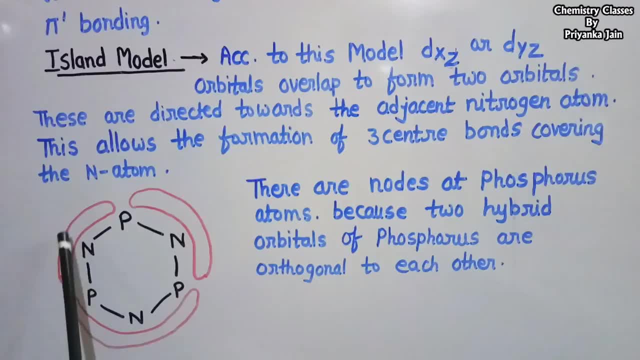 formed. so three centered bond and this nitrogen is also covered in that bond and there will be a node at the phosphorous atom. this is the note you can see. this is the note. this is the rodent, this is the cold. this node is presented, the phosphorus atom. why? because that two hybrid 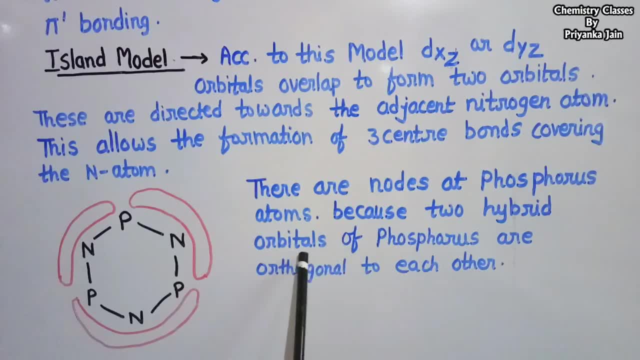 orbitals of the phosphorus that are formed by the overlapping of the xz and the yz orbital. these two orbitals are orthogonal to each other. it means they are perpendicular to each other, so there will be a node. so in this case there will be three nodes. 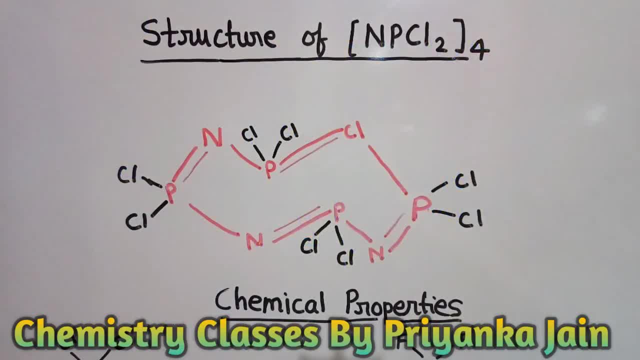 at three phosphorus atom. now we see the structure of the tetramer, that is, octachlorocyclopolyphosphagene, npcl2, whole four. and in this structure this is a tubular structure or tube like structure, and this will be like that. and in this structure there may be two forms. one form is chair form and 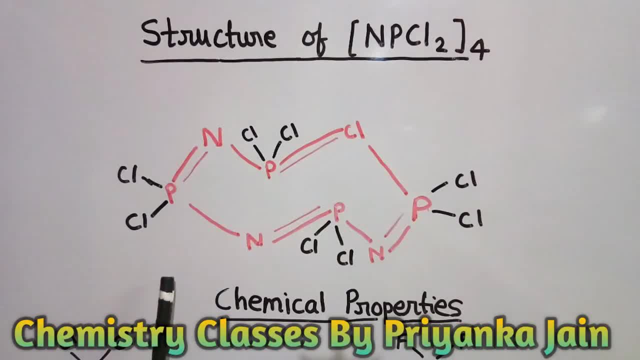 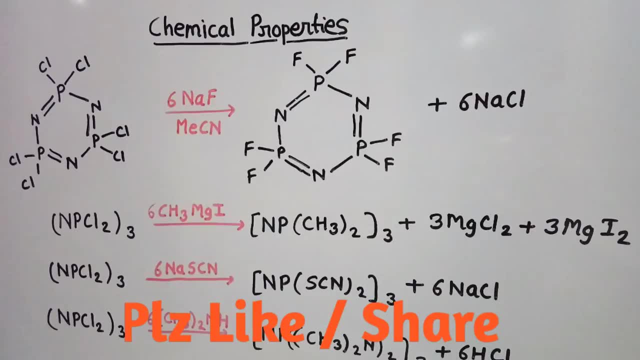 another is both form and the chair. form is obviously the more stable form and this is the structure of npcl2 whole four. now we see the chemical properties of the, especially trimor hexachlorocyclopolyphosphagene. this is the structure of hexachlorocyclopolyphosphagene. 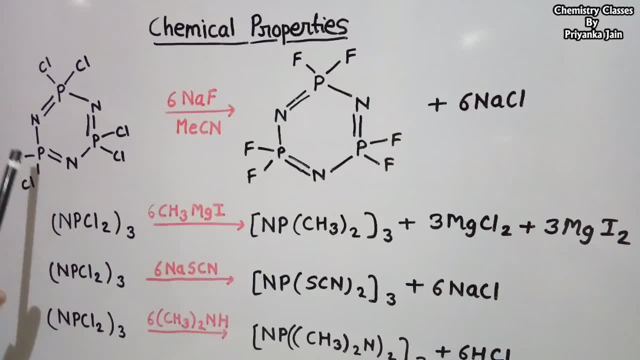 and if we see the properties of this in this structure, the chloride group is reactive and it is replaceable and it can be replaced by the several reagents when they are treated with it. for example, if we get reacted with sodium fluoride, then six molecule of it can react with this and this chloride is replaced by the. 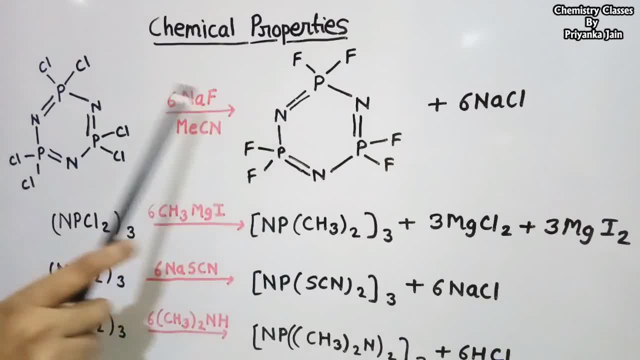 fluoride and this compound is formed. you can see this chlorine is replaced by this floury and the NSE, Alice, formed. similar reaction will take place. we have not made the other structures and we have shown it only by the formula. you can understand it very easily. this CL2 group is replaced every. 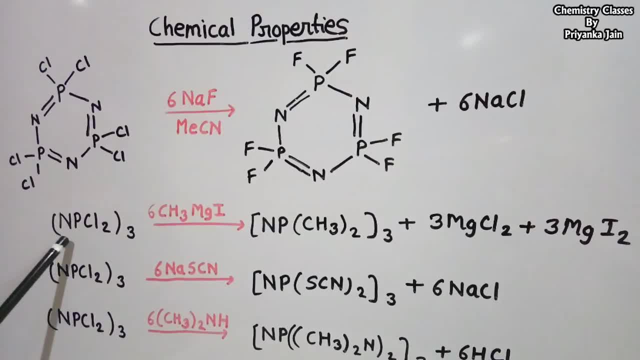 time this chloride groups are replaced. for example, if we reacted with Grignard reason CS3 mgi, the, Then this chloride will be replaced by this CH3 and the compound that is formed is NpCH3 whole twice, then thrice, plus 3 MgCl2 plus 3 MgI2.. 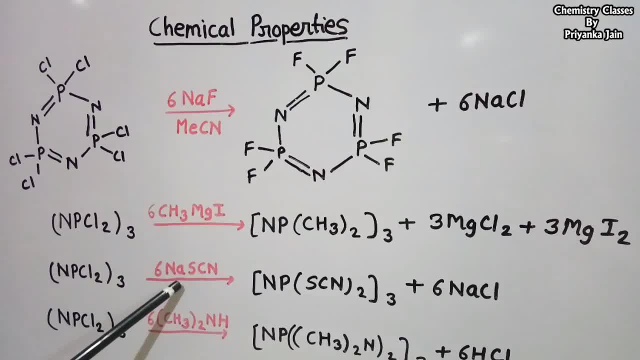 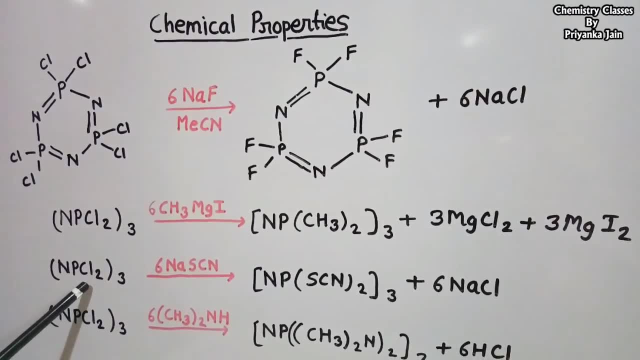 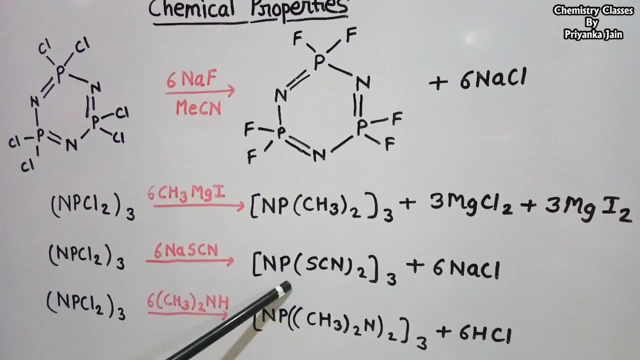 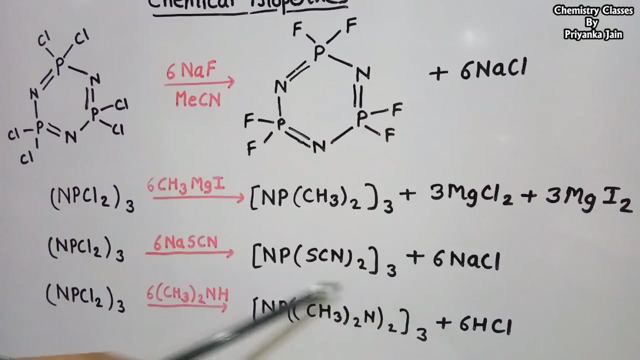 Similarly, if we reacted with the NaSCN, then what happens? this chloride is replaced by this SCN, The 6 atom of chlorine will be replaced by this SCN. it means thiocyanate group and this compound will be formed. and there will be 6 SCN groups here and NaCl will be formed. 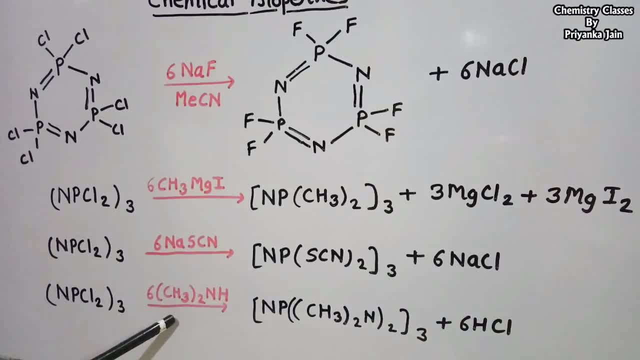 Similarly, if we react this phosphagen with this CH3 whole twice NH, it means this is a secondary amine. and what happens? this dimethylamine group is replaced By this chlorine and the compound is formed NpCH3 whole twice, and then whole thrice plus 6 SCN. 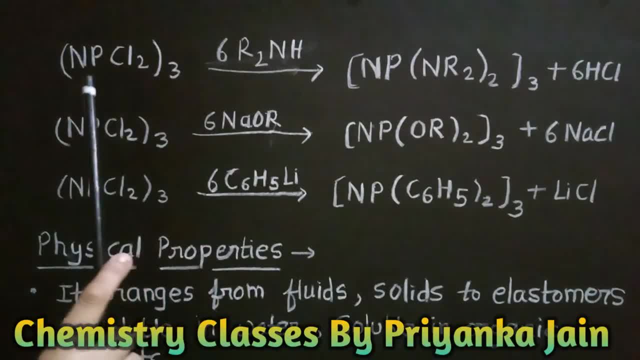 Phosphagen is reacted with R2NH, then what happens? this chloride is replaced by the Nr2 group. and what happens? this is formed: NpNr2- whole twice, then whole thrice plus 6 SCN. Similarly, if this is reacted with NaOr, then what happens? this NaCl is formed. 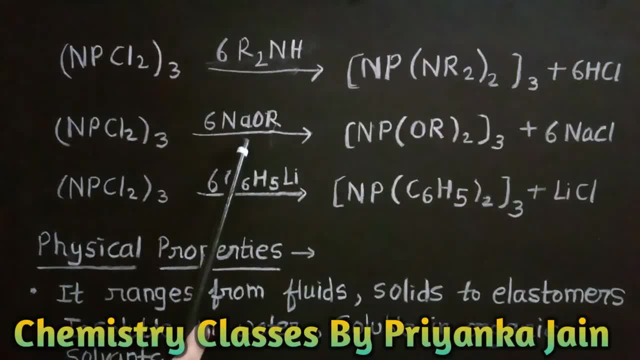 This chloride is replaced by OR group or ethoxy. it may be methoxy, any alkoxy group may be. and what happens? this alkoxy phosphagen is formed Npor2, then whole thrice plus 6 NaCl. Similarly, if it is reacted with C6H5 Li, then this chloride is replaced by the phenyl group and NpC6H5- whole twice, then whole thrice. 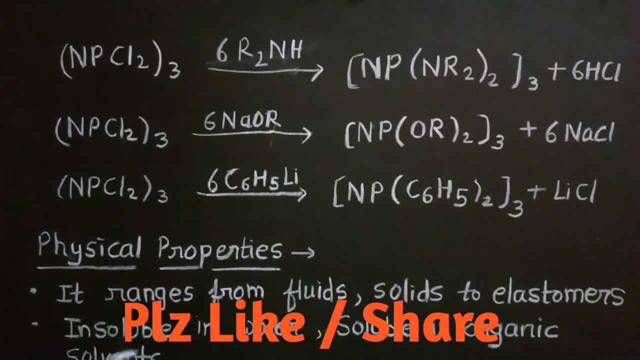 Similarly, if it is reacted with C6H5 Li, then this chloride is replaced by the phenyl group and NpC6H5 whole twice, then whole thrice, plus 6 NaCl. If we look at the physical properties of the phosphagen, 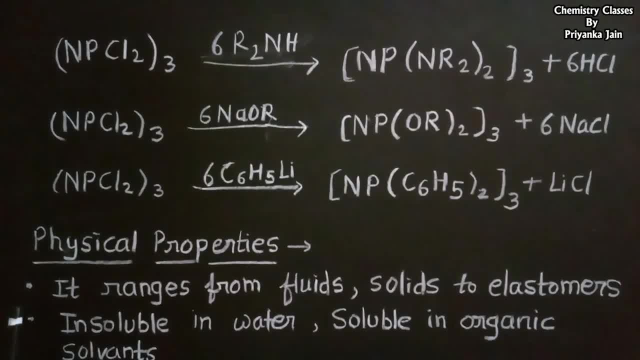 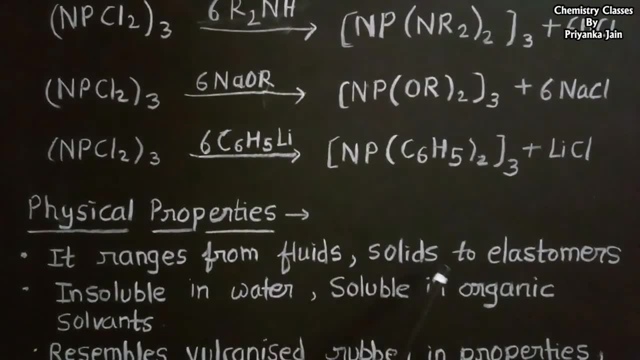 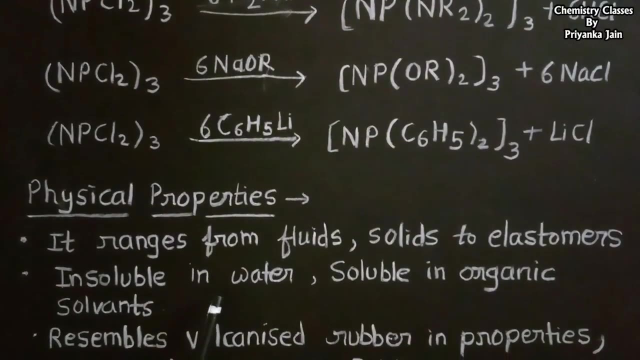 The phosphagen forms a high range of compound. a very large number of compounds are known, And it ranges from flutes to solids and then to elastomers. it means it may be flutes, they may be solids or they may be elastomers, And these are insoluble in water and soluble in the organic solvents. 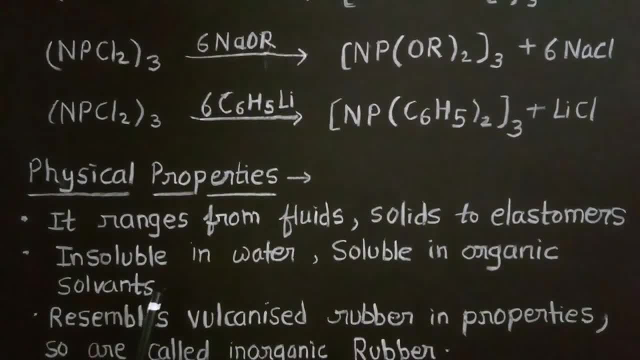 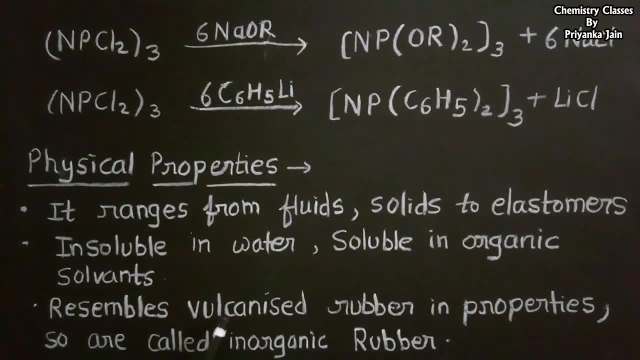 And these are insoluble in water and soluble in the organic solvents. But in the case of higher molecular weight, phosphagen, they are insoluble in the organic solvents also And these resembles the vulcanized rubber in the properties. Its properties are similar to that of the vulcanized rubber.